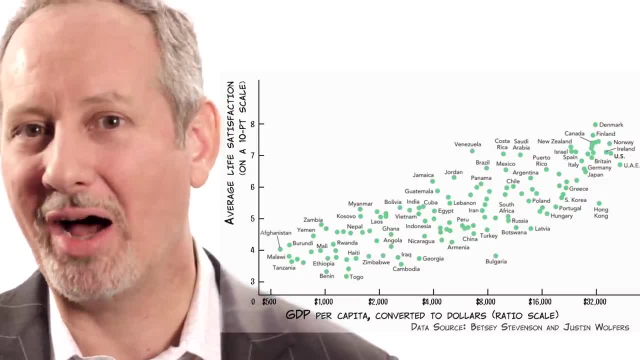 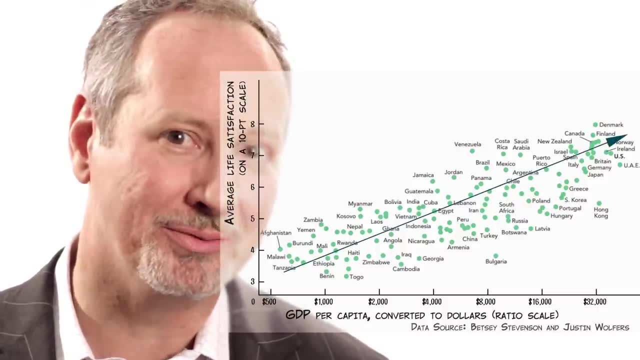 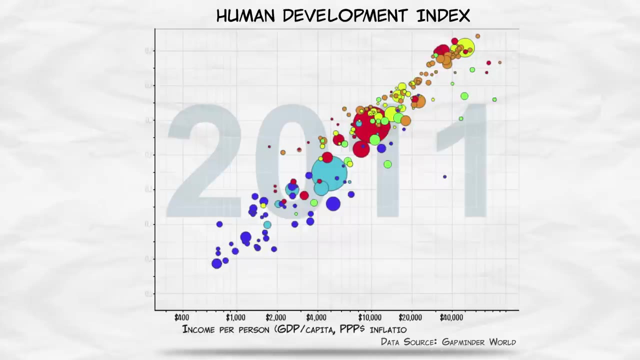 on the vertical axis, Again we see a positive correlation. Countries with a higher real GDP per capita also tend to have happier people on average. Here's a data set from the United Nations. It's called the Human Development Index. It combines measures of life expectancy, education, 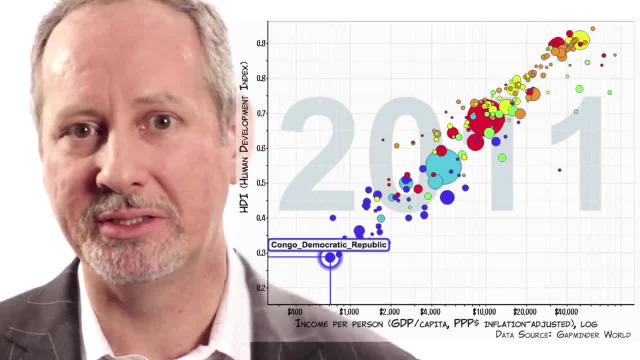 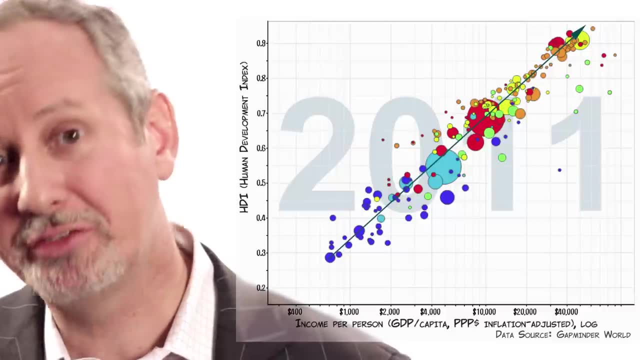 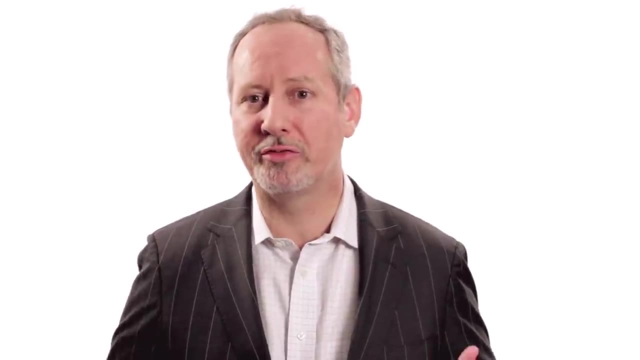 and standard of living Overall. you can see, in general, as GDP per capita increases, so does human development, at least as measured by this index. The basic story, it's pretty simple: When we have more goods and services, we can usually afford more of the other good things in life. 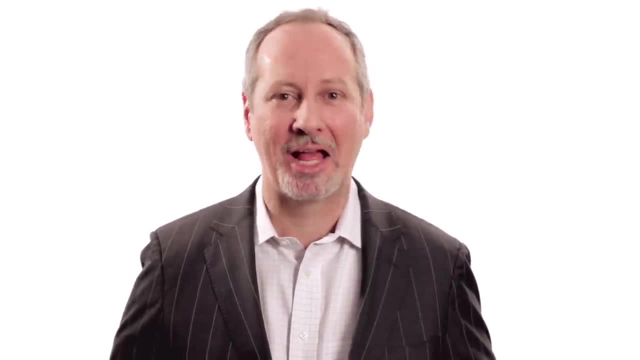 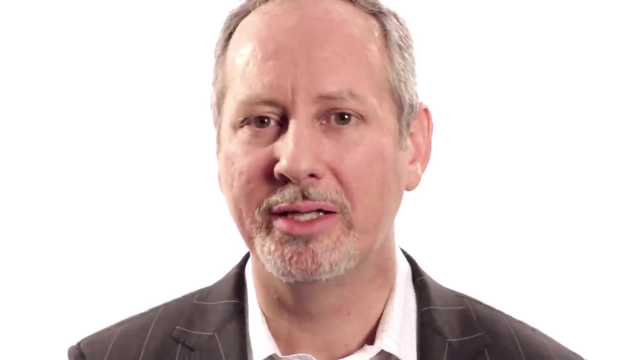 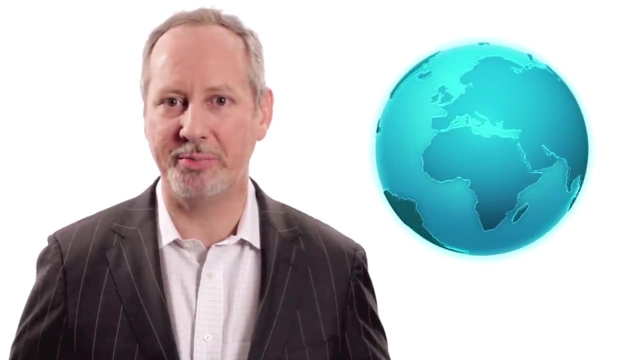 So the good things in life. they tend to go together. However, GDP per capita is far from perfect. Here's one problem: GDP per capita misses the distribution of income. For example, let's compare the real GDP per capita of Nigeria, Pakistan and Honduras. 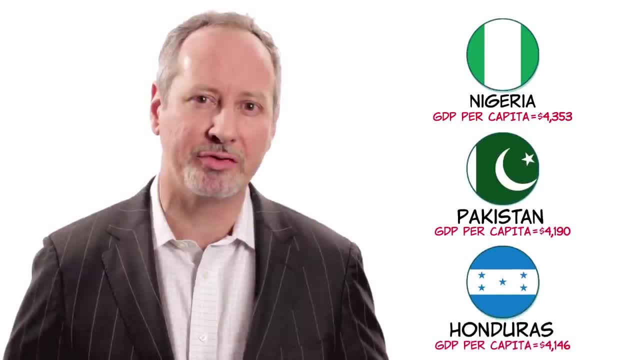 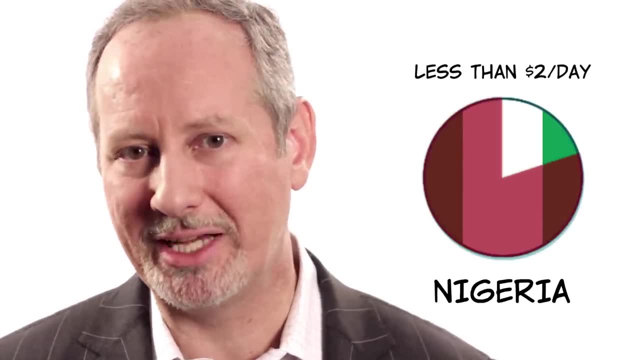 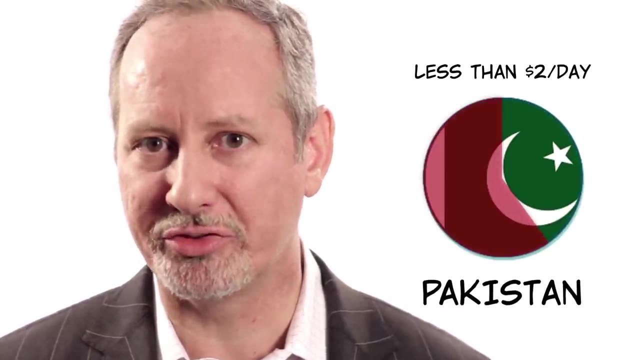 It's actually pretty similar, So you might think that all three countries have similar living standards, And yet in Nigeria, about 80% of the population lives on less than $2 a day. In Pakistan, it's only 60%. In Honduras, it's only 33%. 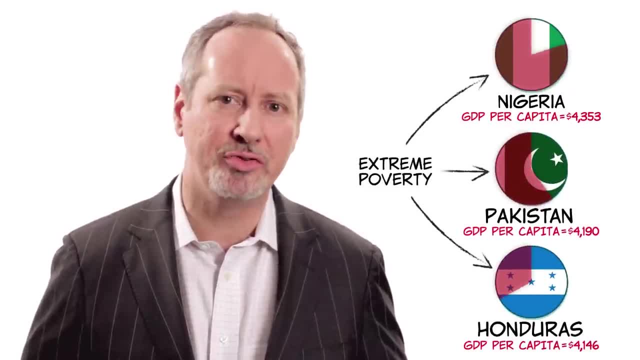 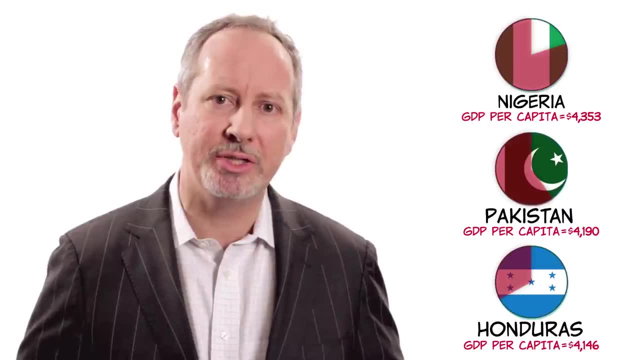 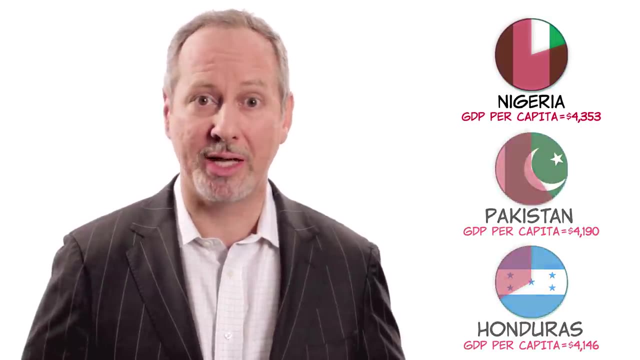 How can the number of people living in abject poverty be so different when real GDP per capita is about the same? The reason is that income in Nigeria is much more unequally distributed than in Pakistan or Honduras. Nigeria has many poor people, but also some very rich people. 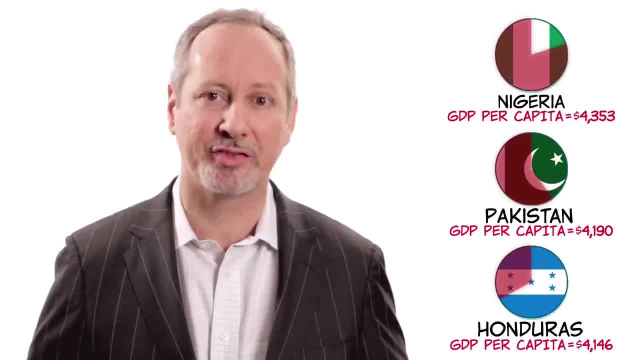 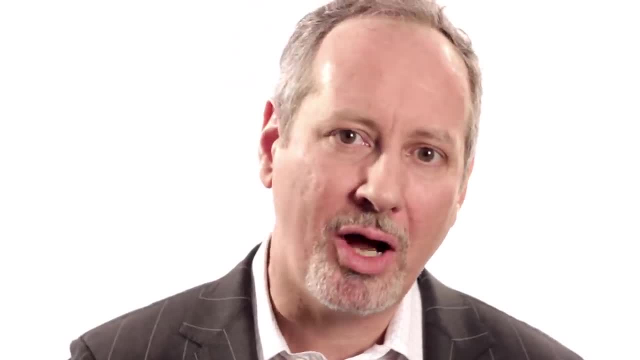 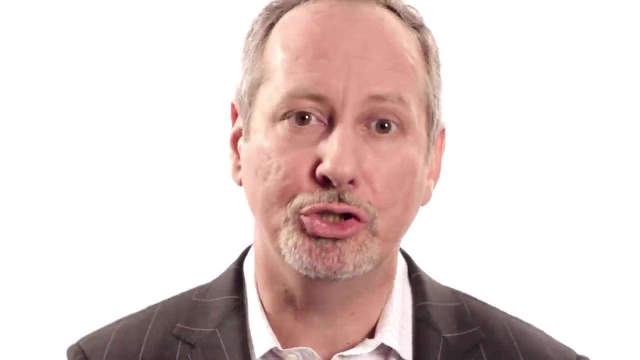 So average income it's about the same in Nigeria, Pakistan or Honduras, even though there are more poor people in Nigeria. Over time, however, growth in real GDP per capita, whether in Nigeria, Pakistan or Honduras, usually does indicate growth in everyone's incomes.